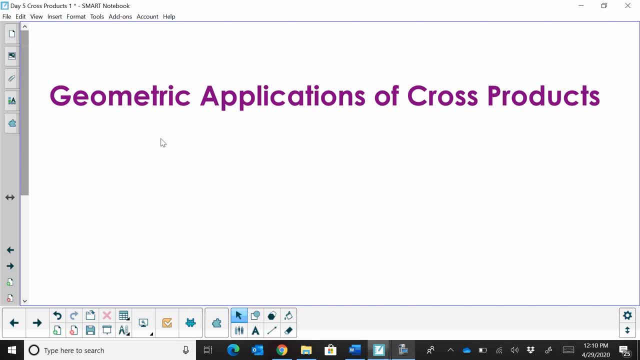 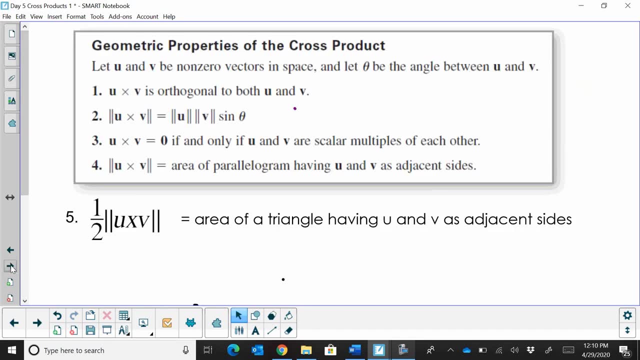 Hi, welcome to MooMooMath. Today we're going to look at geometric applications of cross products with vectors. So let's first look at geometric properties of cross products. So let u and v be non-zero vectors in space. Let's let theta be an angle between the two vectors. 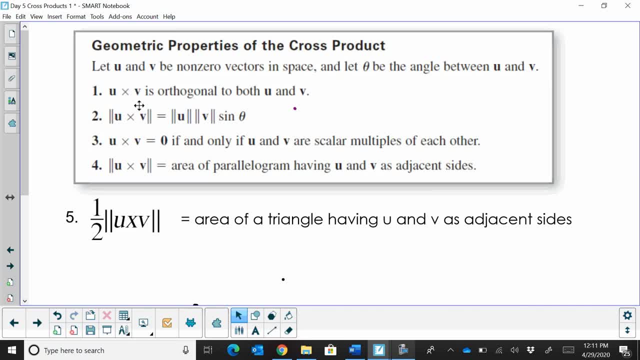 u with a cross product of v is orthogonal to both meaning. when we find the cross product of these two vectors, the result is perpendicular to both of the vectors. Number two: the magnitude of the resulting vector from the cross product is equal to the magnitude. 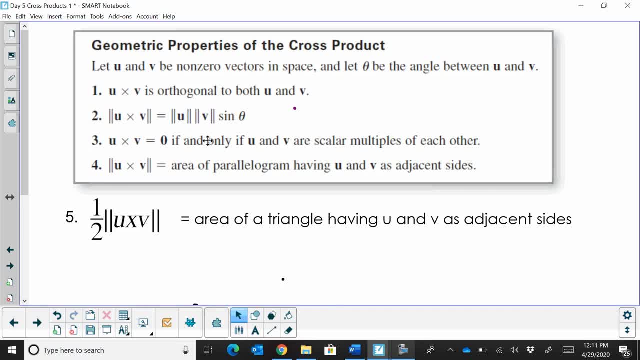 of u times the magnitude of v times the sine of theta, and theta is the angle between the two vectors. The third property would be when you find the cross product and you get zero. that means u and v are scalar multiples of each other, meaning they are parallel to each other. So the only way 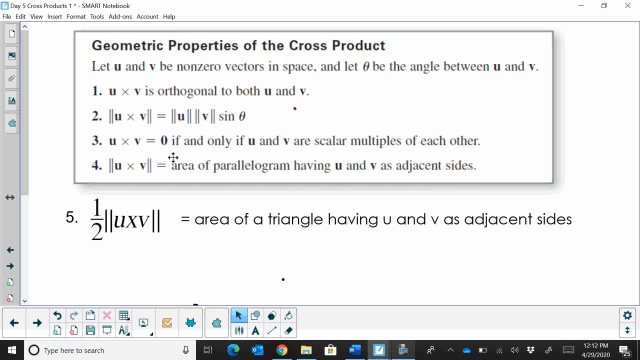 for them to be scalar, multiples, or they're parallel. therefore, there isn't a vector that's perpendicular to both because they're not. they're parallel. therefore, there can't be a vector that's perpendicular to both because they're parallel to each other. And the fourth one is when you find 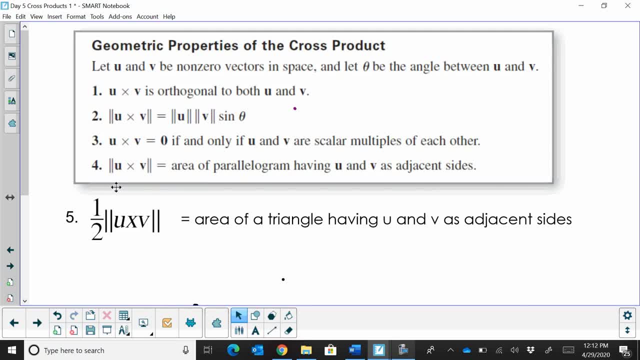 the cross product of u and v and you get that resulting vector. once you find the magnitude of that resultant vector, you're going to be able to find the cross product of u and v. So that's equal to the area of a parallelogram having the two sides of u and v as the adjacent. 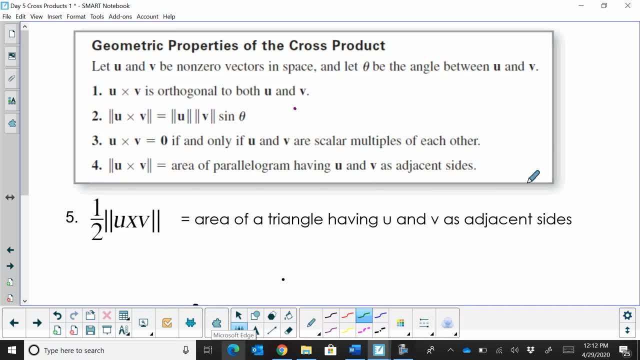 sides of a vector. So if you have two vectors, I'll just kind of sketch that. So if you have two vectors in three dimensions, if you extended that into a parallelogram, that would be the area, And then of course I added a fifth one, If you have, and it just 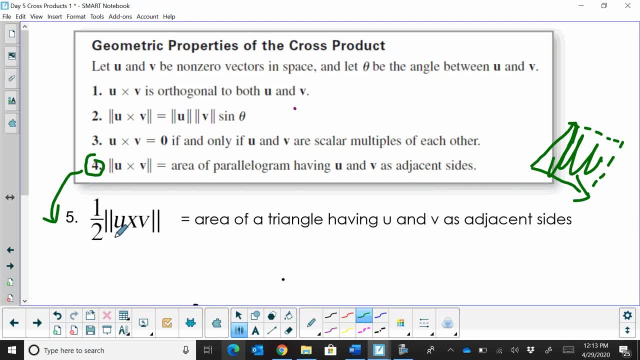 ties into this fourth one. If you find the magnitude of the resulting vector of the cross product, you take half of that magnitude. that equals the area of a triangle having the two sides. So basically, you're looking at the same vector but you're just looking at half of it. 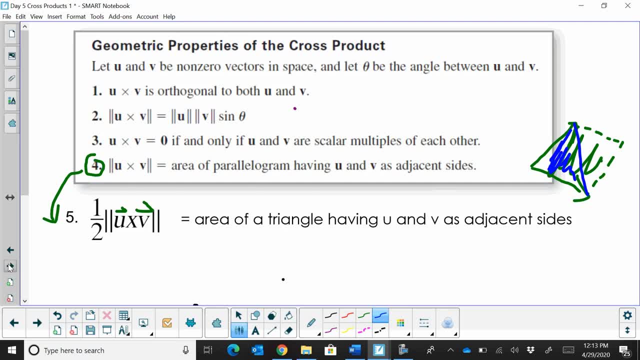 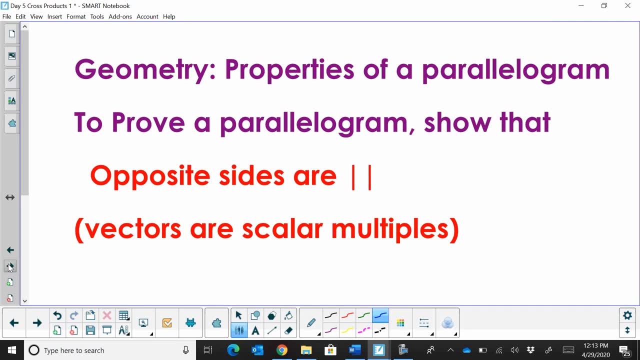 to find the area of the triangle in three dimensions. So let's look at some proofs and things we can do with geometry. So in geometry we know one of the properties of a parallelogram is the opposite sides are parallel. So in three dimensions we can use vectors to prove a parallelogram. We would just 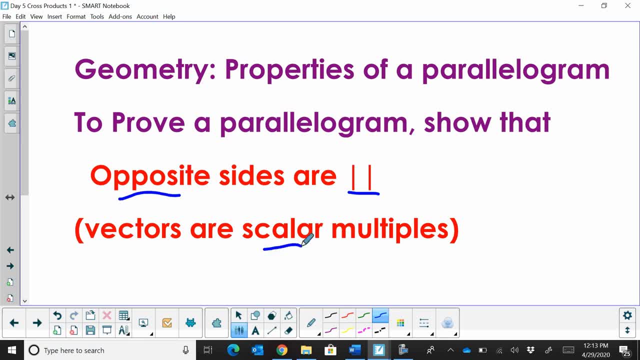 show that the opposite sides are parallel, showing their scalar multiples of each other. So if you find that these two sides are scalar multiples and these two sides are scalar multiples, comparing both pairs of sides, you could then say you had a parallelogram in three dimensions. 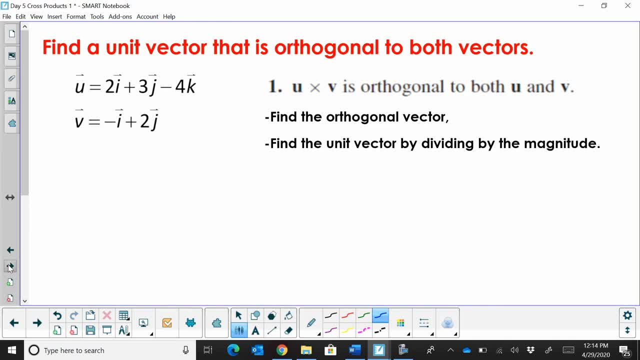 Okay, we're going to start by working some problems looking at unit vectors, that unit vector that's orthogonal to both vectors. So I'm given vector u and vector v and I want to find a vector that is orthogonal to both. Well, in order to do that, I can just find a cross product and I 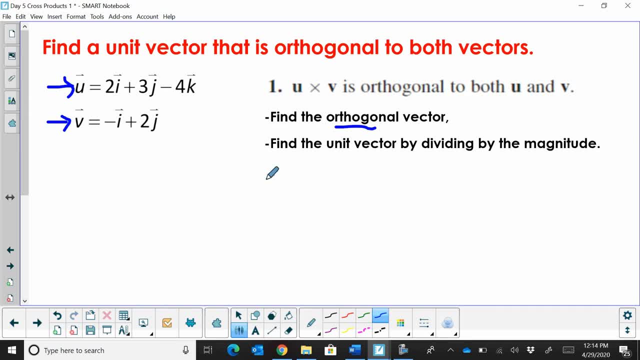 know that that vector is the is orthogonal to both. Then, once I find that vector, I can write it as a unit vector by just dividing by the magnitude. So let's first start with our cross products. So, finding the vector that's orthogonal to both, I'm going to draw out to create my cross product. I'm going to take 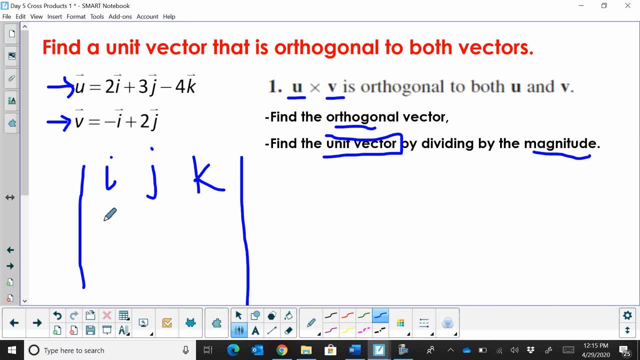 u times v. So u is going to go first: 2, 3, negative 4, v, i, j and k must be 0.. So negative 1, 2, and 0.. To find this cross product, I'm going to take the coefficient for i, which would be 0 minus. 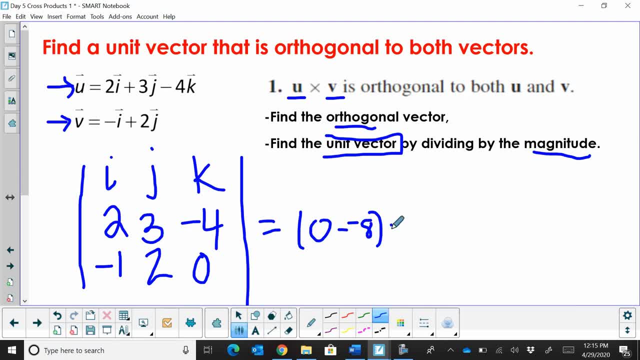 negative 8, i Minus the j, which would be 0 minus 4j, plus the coefficient for k would be 4 minus a negative 3.. So my vector would then be 8, i Minus the negative 4, so plus 4j, and this is going to be plus 7k. 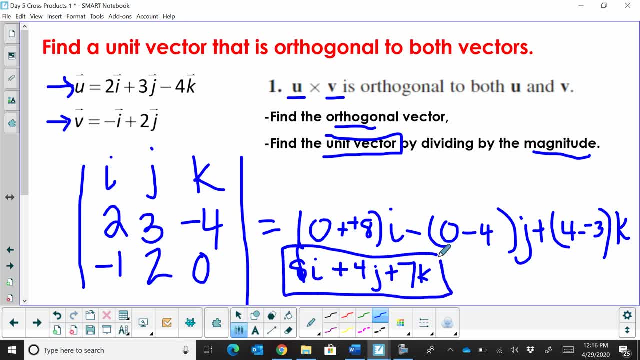 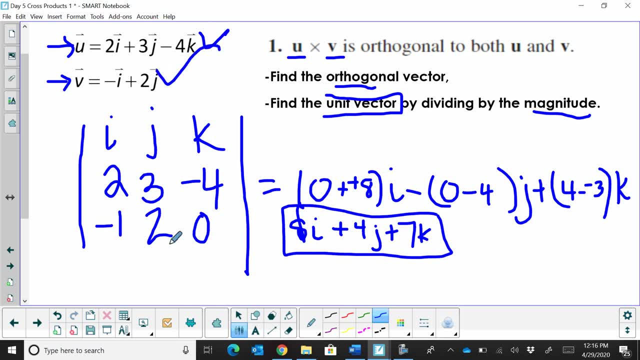 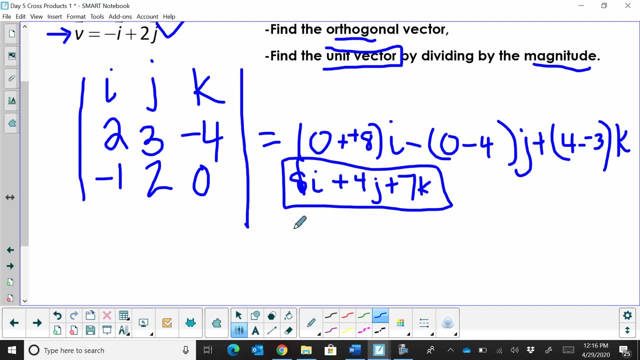 So there is my cross product, that the vector created that is orthogonal or perpendicular to the two given vectors. Now I want to find the unit vector. So to find the unit vector for this vector, I have first got to find the unit vector for this vector. So I'm going to take the unit vector and I'm going to 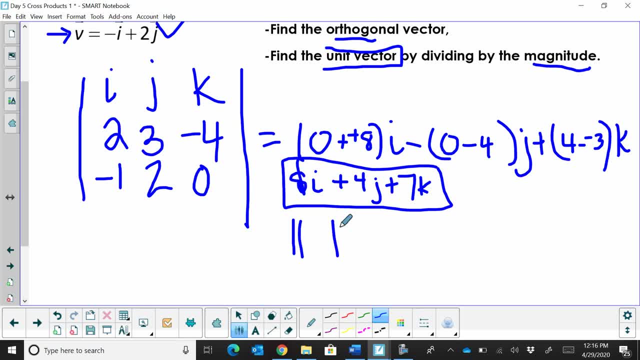 find the magnitude, So let's take the magnitude of. I'll call this a vector z. No, not z, because we're using that. Let's call it vector w. I'm going to find the magnitude of w, So I'm going to take 8. 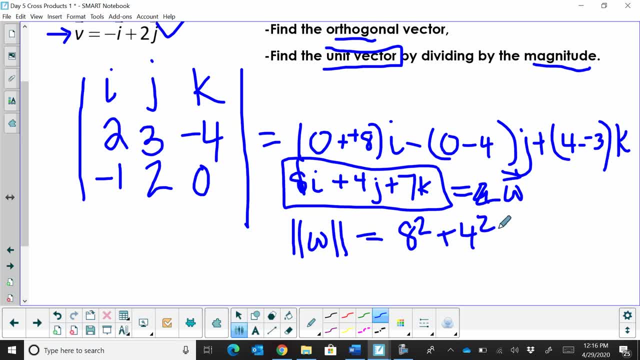 squared plus 4 squared plus 7 squared, and take the square root of that, So that's 64, plus 16,, which is 80.. 80 plus 49 is 129.. So I'm going to take the square root of 129.. 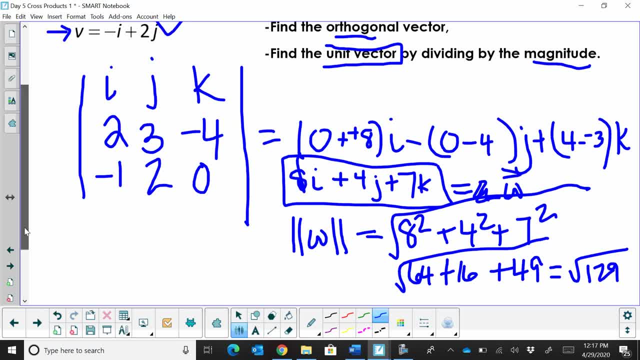 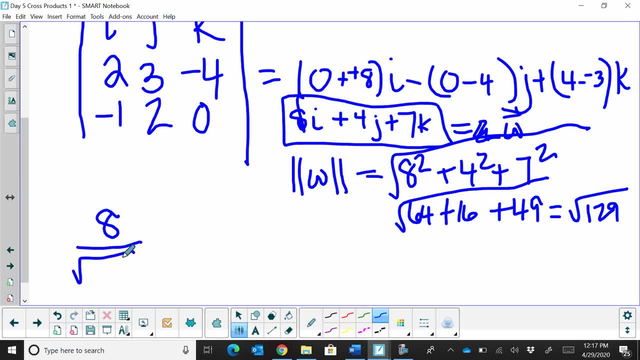 That is my magnitude. Now to write the unit vector, I'm going to take the vector and I'm going to divide it by the magnitude. So that's going to be 8, 8 over root 29i, plus 4 over root 129j, plus 7 over root 129k, And we can do a little cleaning. 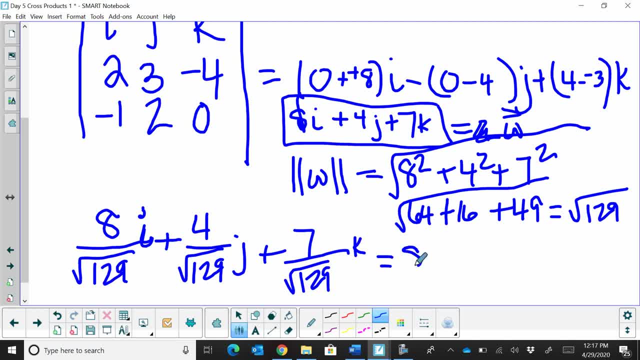 up just to not have a radical in the denominator, And we know that's 8 root 129 over 129.. By multiplying top numerator and denominator by root 29i plus 4 square root 129 over 129j, plus 7 root 129 over 129k, And that would represent the unit vector that is. 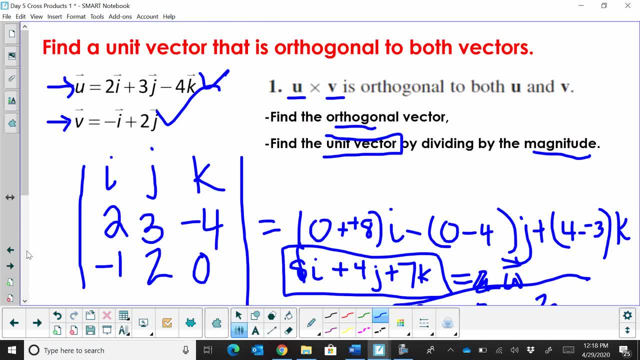 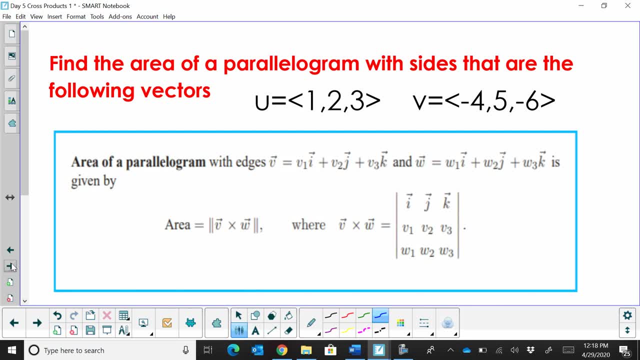 orthogonal. So that's the unit vector that is orthogonal to the two given vectors. So now let's look at the application of finding the area of a parallelogram with sides that are given as the following vectors: We have the vectors 1,, 2,, 3, and vector v, which is: 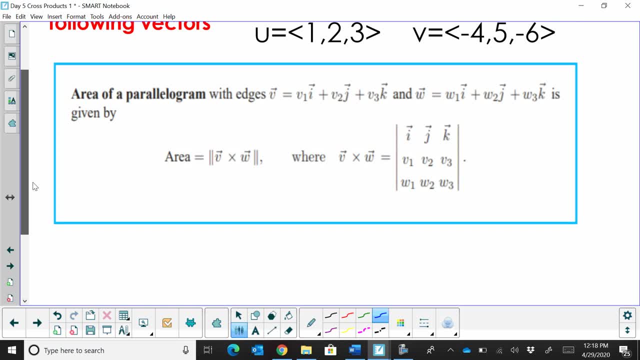 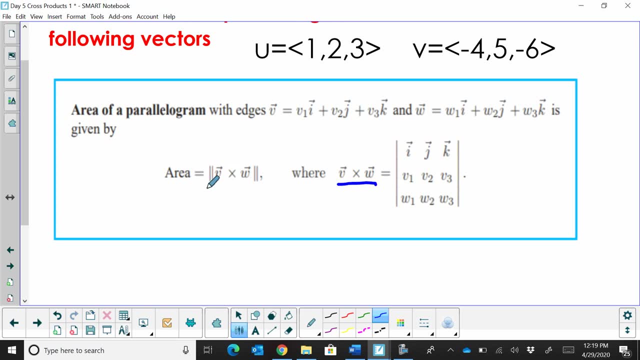 negative 4, 5, and negative 6.. And we want to find the area of the vector. All we need to do is first find the cross product, Then we're going to take the magnitude of that answer. So let's start off by taking u times, w or v. in this case, We're just going to 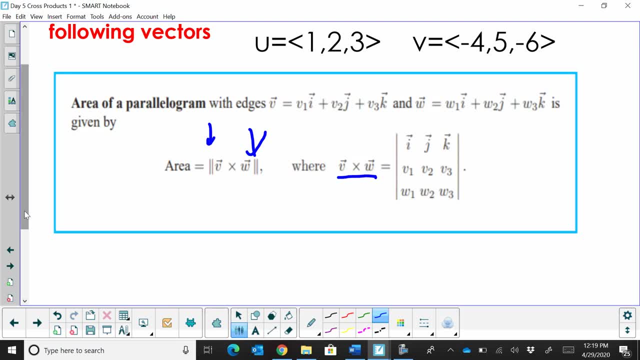 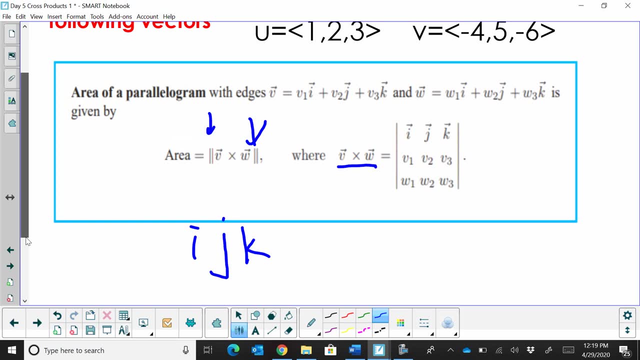 these variables are different, but we're using the same thing. So let's start with our i, j, k, i, j and k, And the first one is just 1,, 2, and 3.. That's our first vector. Our second vector: 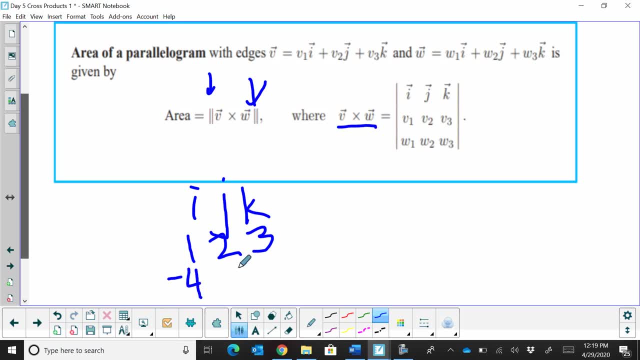 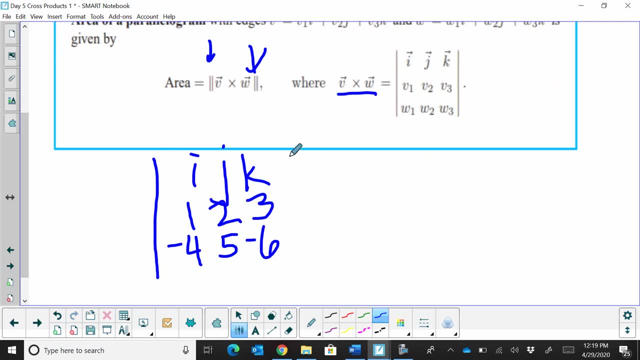 is negative 4,, 5,, 6.. And I believe that was supposed to be negative 6.. Yeah, Let's expand this. So our coefficient for i is negative 12 minus 15. i minus for j. I'm going to get a. 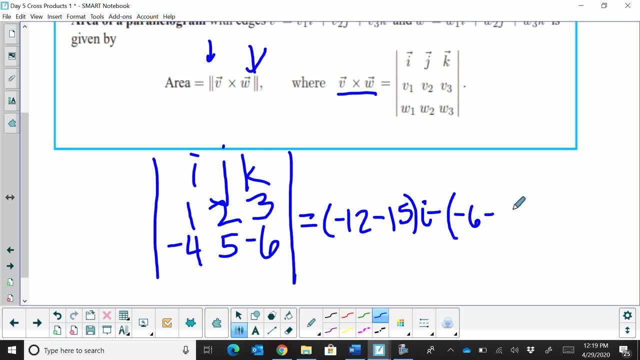 negative 6 minus negative 12 plus that's j plus the coefficient for k would be 5 minus a negative 8. Ends up being a positive. We're going to add those, So let's see We have negative 27 i. 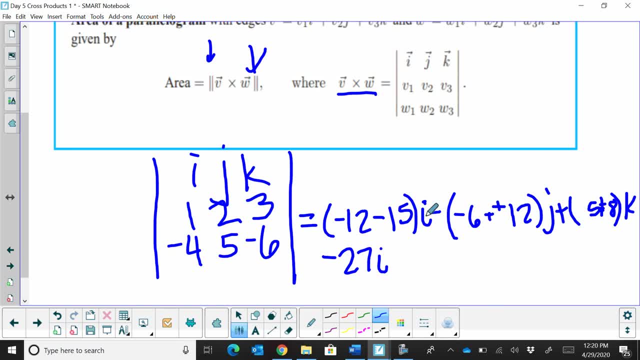 double negative. here That's going to be 6.. So minus 6 j And over here I've got a positive 13 k. So there is my cross product. Now I need to find the magnitude of this cross product, So I'm going to have to use a calculator. 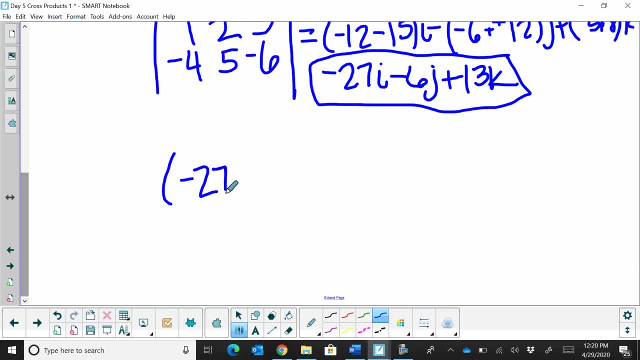 on this one. So negative 27 squared plus negative 6 squared Plus 13 squared And I'm going to take the square root of all that to find the magnitude. So let's grab a calculator, Let's see. It's going to take a little more than I can do in my head. 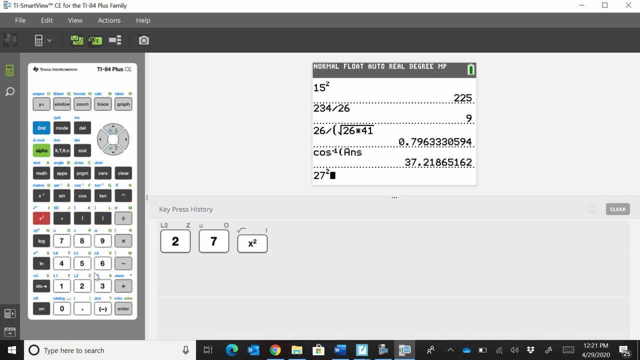 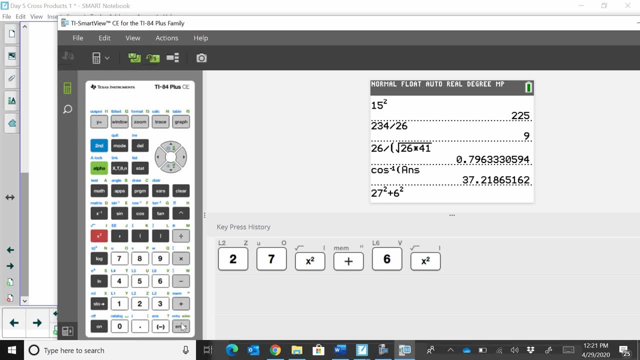 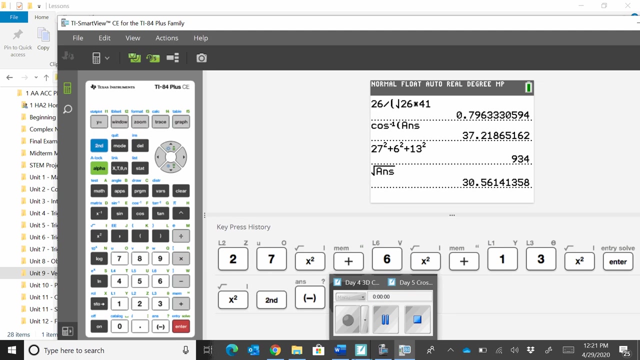 So that gives me 27 squared plus 6 and 13.. 6 squared and 13 squared And let's take the square root of that answer And that's going to give us 30.56.. 6.. Let's get back to my smart board here. 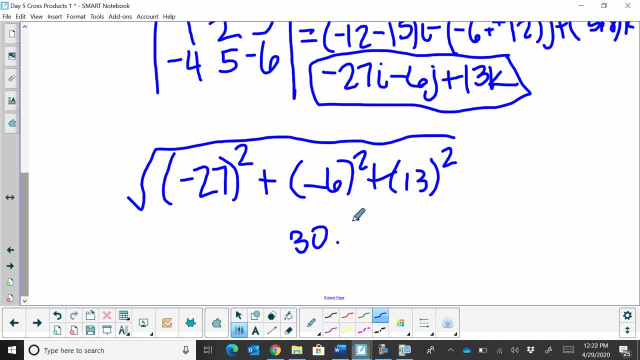 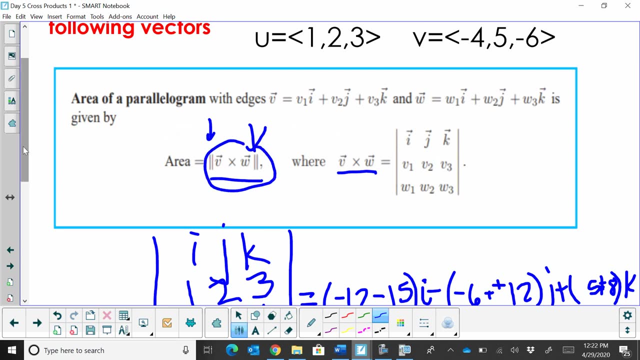 So that's 30.56 square units. So that's how I find the area of a parallelogram. It's just simply find the cross products vector and then find the magnitude of that vector, And there we go, Which is the distance. 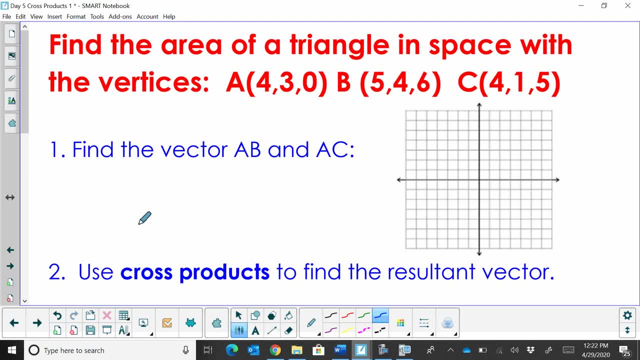 Now let's find the area of a triangle in space with the vertices 4, 3, 0.. 5, 4, 6. And 4, 1, 3 as those three vertices. So the first thing we want to do is find the resulting vector for vector AB. 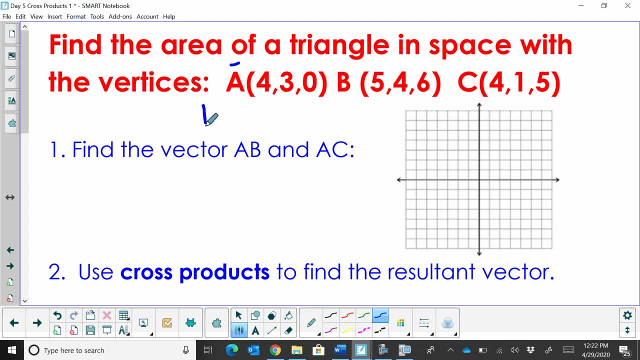 So to find the resulting vector, I'm going to do terminal Terminal minus initial. Remember, these are just points out in space So I have to write them as vectors. So from A to B, So terminal minus initial. 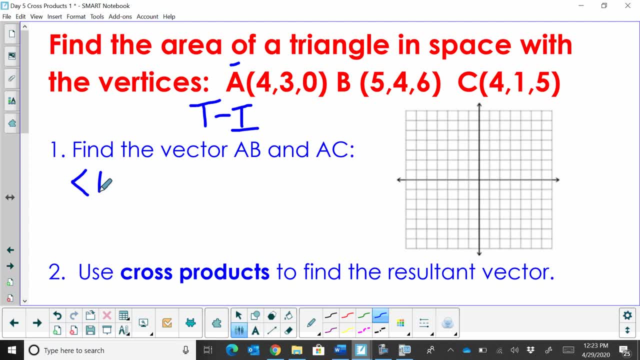 I'm going to take 5 minus 4,, which is 1.. 4 minus 3,, which is 1., And 6 minus 0,, which is 6.. So there is the vector AB, AB, AB as AB. 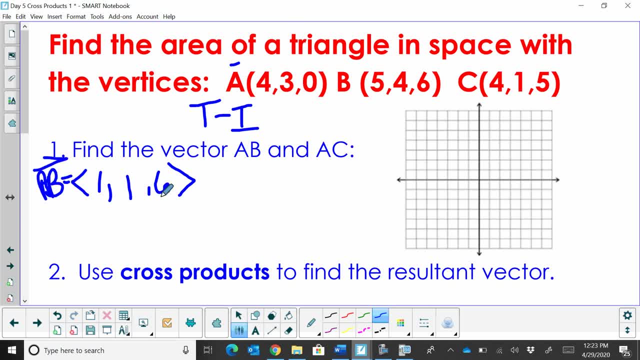 Remember it's terminal minus initial, And I'm going to find the vector AC Again. I'm going to do the same thing. I'm going to take terminal, which is C, and subtract A from it. So 4 minus 4 is 0.. 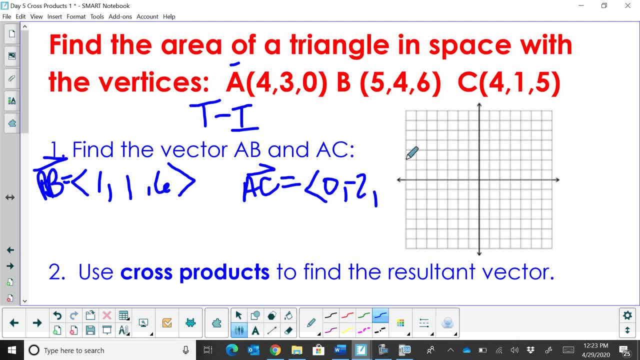 1 minus 3 is negative 2. And 5 minus 0 is 5.. So there is my second vector. So I know that these, These two vectors are connected. at A. They both radiate out of the point A, because I went from A to B and A to C. 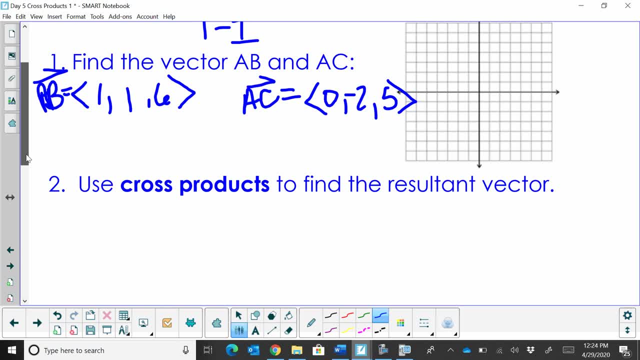 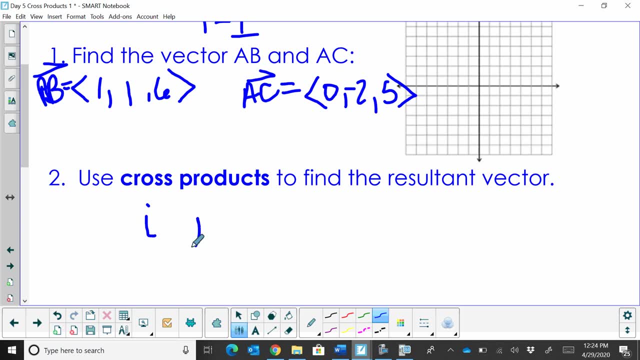 Now, that's your first step. You just find the vector. Now we want to find the cross product of that vector. So I, J K And I'm going to take AB first. So 1, 1,, 6.. 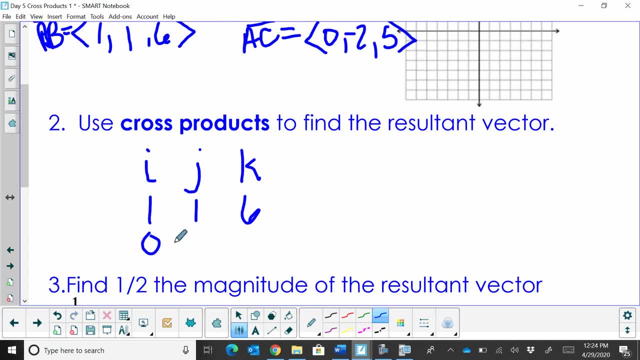 I'll take AC, second: 0, negative 2, 5.. Let's first find the resulting vector from expanding it. So my coefficient for I would be 5 minus a negative 12.. So that's going to give me 17I minus. 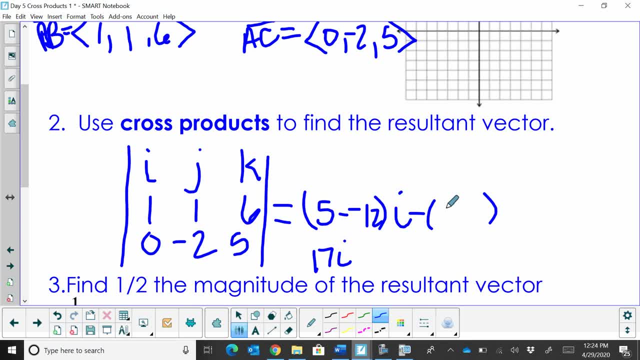 Minus Coefficient for J would be 5 minus 0.. For J- So that's just going to be minus 5J plus K- The coefficient for K would be negative 2, also minus 0. So that's just going to be minus 2K. 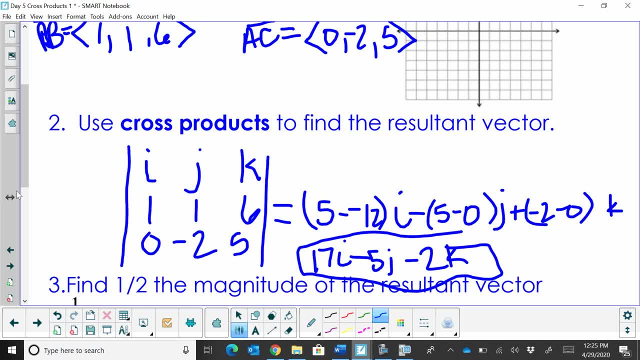 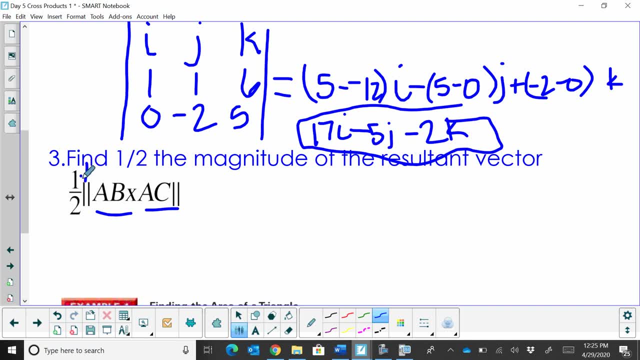 So there is my resulting vector. Now I need to find the magnitude. So once I multiply these two vectors together, I find the negative 2.. So that's just going to be minus 2.. I find the magnitude and then for a triangle I'm going to take half of that. 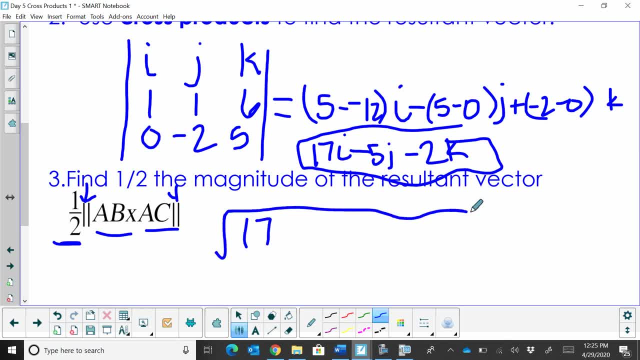 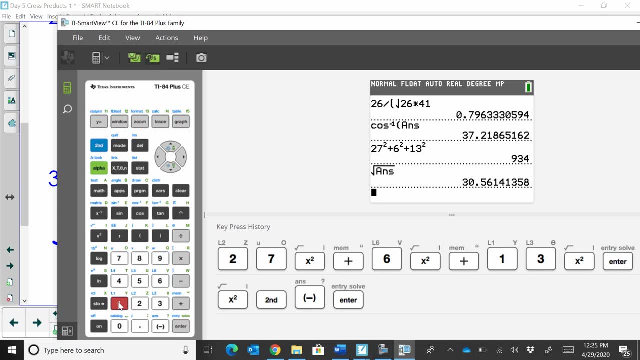 So let's find the magnitude 17,. that's the square root of 17 squared, plus negative 5 squared, plus negative 2 squared, And 17 squared, I believe, is 289.. Let's just double check my math: 289, yep. 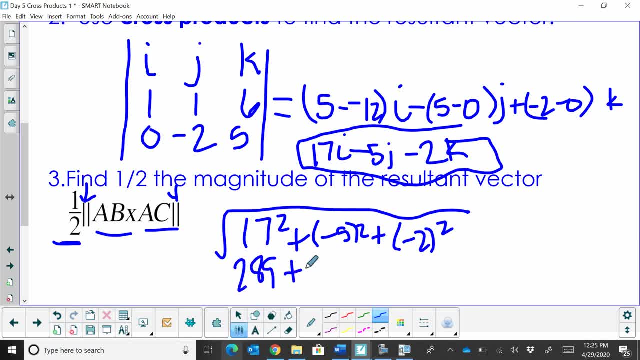 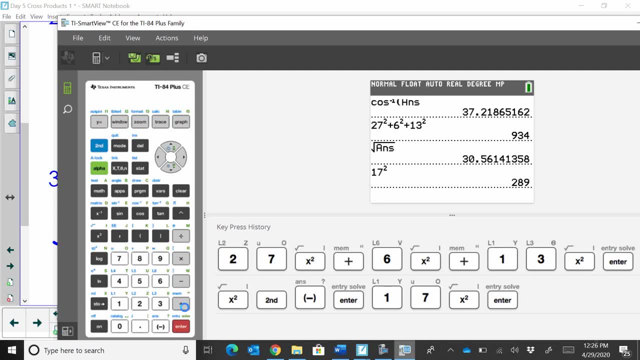 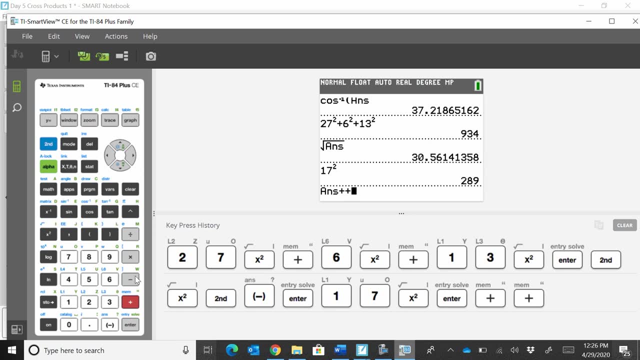 So 289 plus 25 plus 4.. So 289 plus. let's just add 29 to that. My screen glitched for a second. There we go, 318.. And the square root Of 318 is going to give me my magnitude. 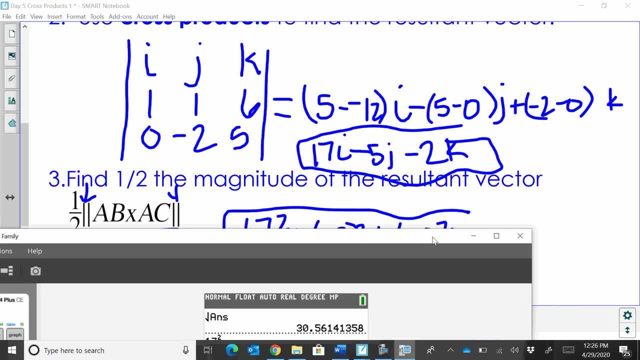 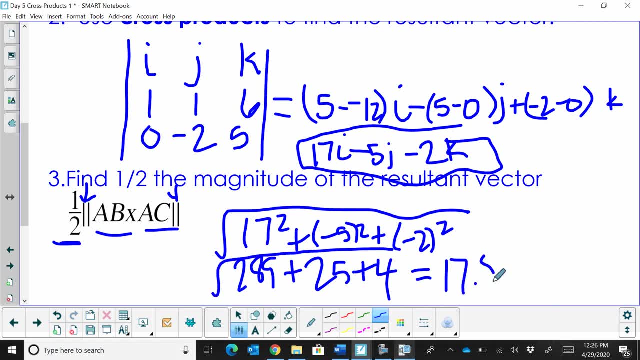 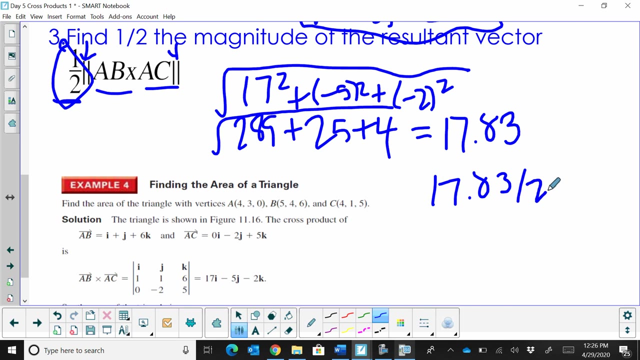 So 17.83.. So 17.83. And that would be the magnitude, but I need to take half of it. So I'm going to take this and divide it by 2.. So 17.83 divided by 2.. 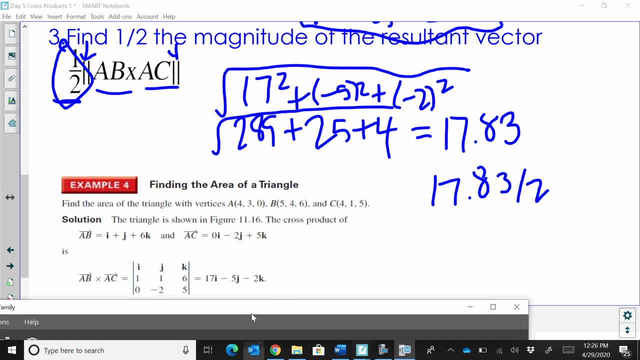 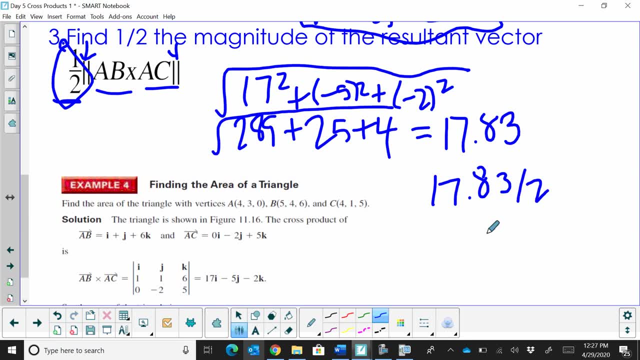 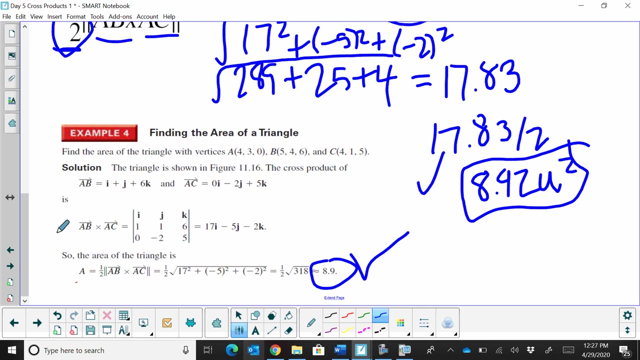 And that will give me the area, So 88.92.. And that will be in square units. And let's just double check our work. Make sure it all looks right. Yes, it looks right, And that's how you find the area of a triangle. 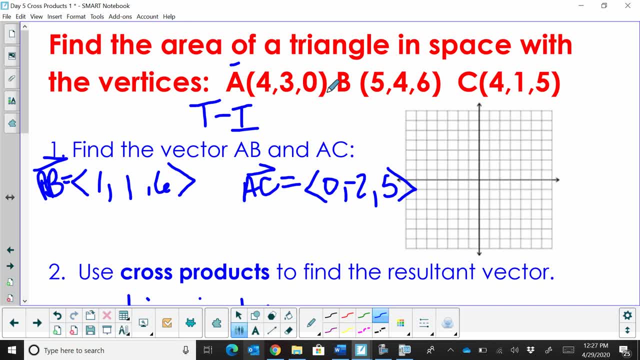 Given 3-dimensional, And that's how you find the area of a triangle. So the first thing you have to do is you have to write the vectors to find two adjacent sides. This is a little bit easier on a triangle because you don't have to worry about if the sides are opposite from each other. 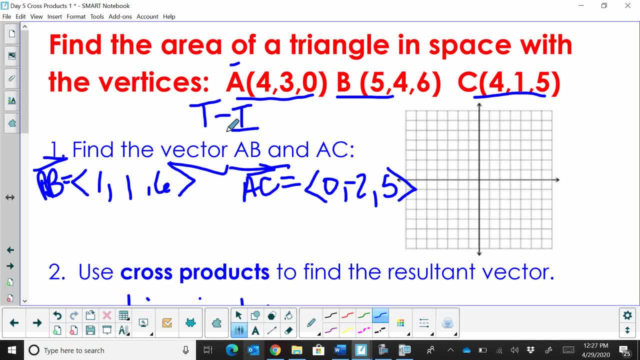 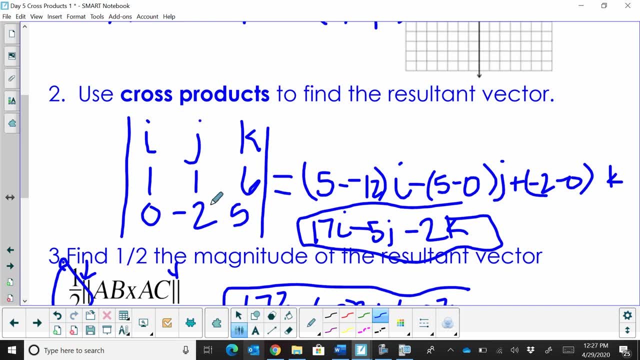 It doesn't matter which vertex you start at. I started at A and found B to A and C to A for my terminal minus initial. Then I found the cross product of the vector And that was a vector. Then you find the magnitude of the vector. 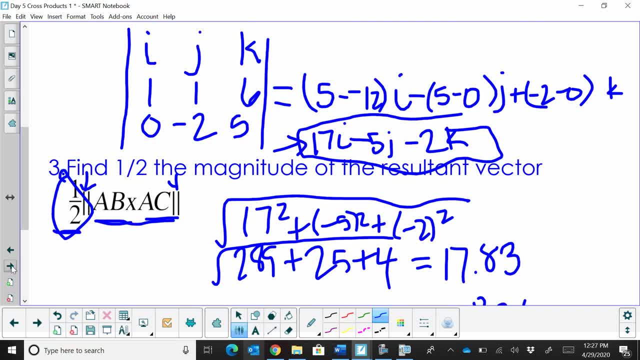 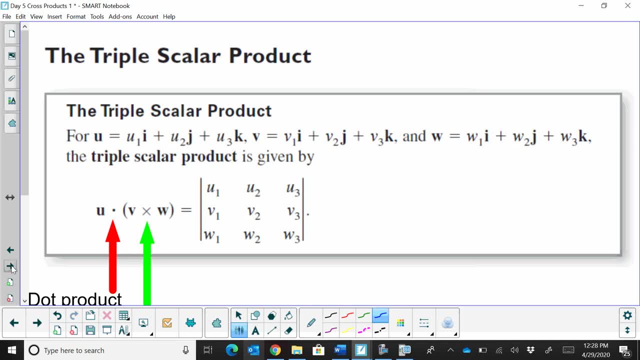 And then you take half of that vector and then you take half of it for a triangle, Okay. So let's talk about the triple scalar product. A triple scalar product is very, very simple. Okay, You are just taking the dot product of a cross product. 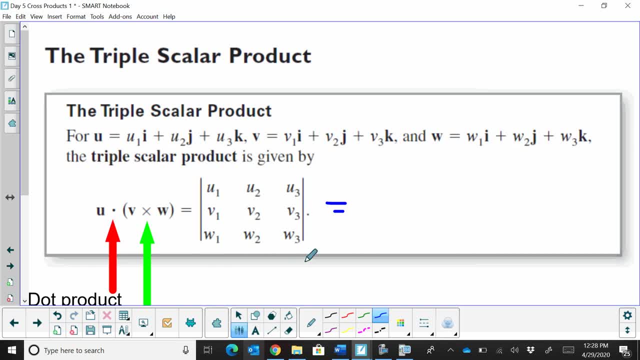 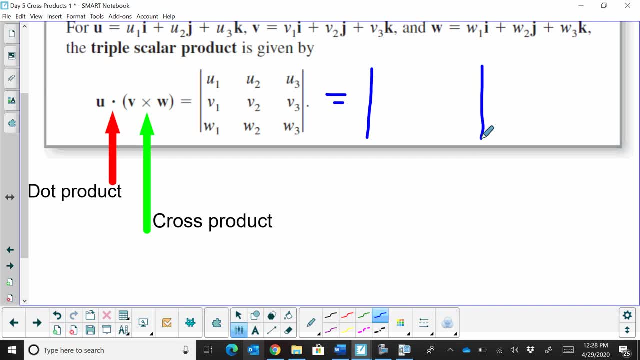 And again, the simplest way is just what we call a triple scalar. So we're going to take the coordinates for each vector and just set them up in each row, And then we're going to find the determinant of that 3x3 matrix. 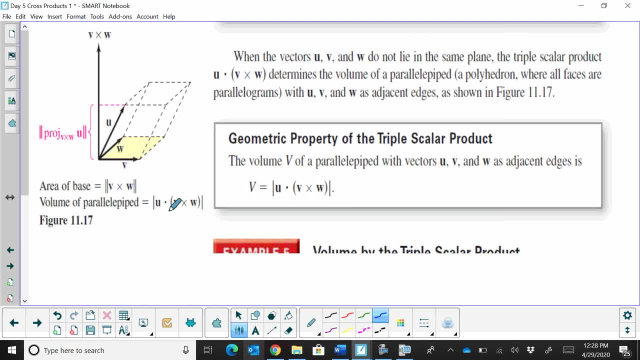 So an application, a geometric property of a triple scalar is very simple. If we have three vectors and they are in component form, we can set them up into this triple scaler, And what it does is it gives us the volume of this three-dimensional shape And this three-dimensional 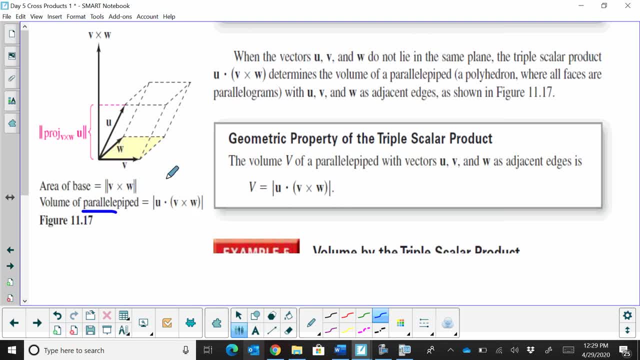 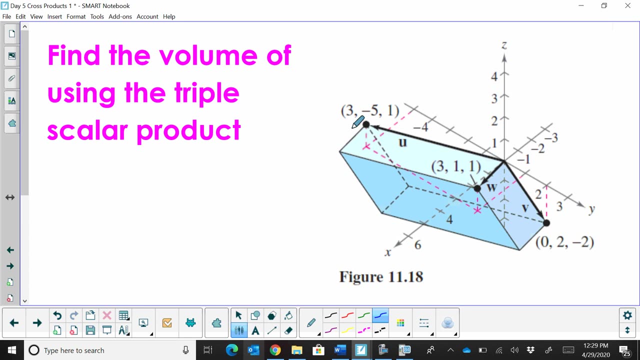 shape is called a parallel pipe. Okay, And that is the volume. So once we do this triple scaler, it's the volume of that three-dimensional figure, which is very cool. So let's try this. We've got three vectors here. All of them are written. well, we're going to write them in. 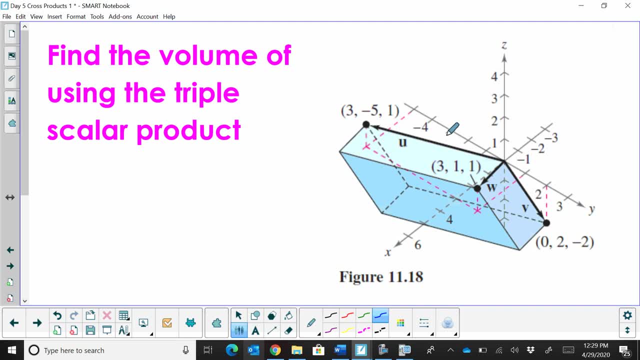 component form. So this position or this point is 3, negative 5, 1.. So since it's being generated from the origin, I can write that as the vector: 3, negative 5, 1.. My second vector is being: is at the point or the 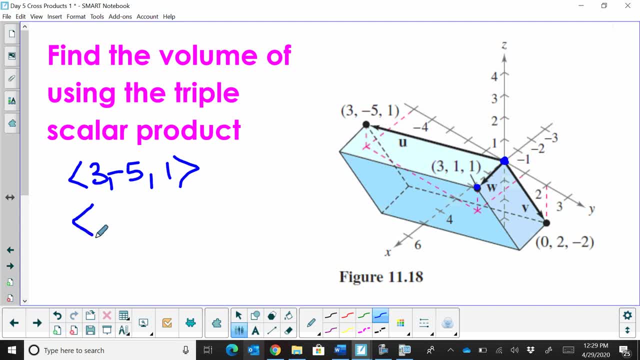 vertex of this three-dimensional figure is at the point 3,, 1,, 1.. So I can write that as a vector, because that side is a vector And this third one is a vector at 0,, 2, negative 2.. And it is the. 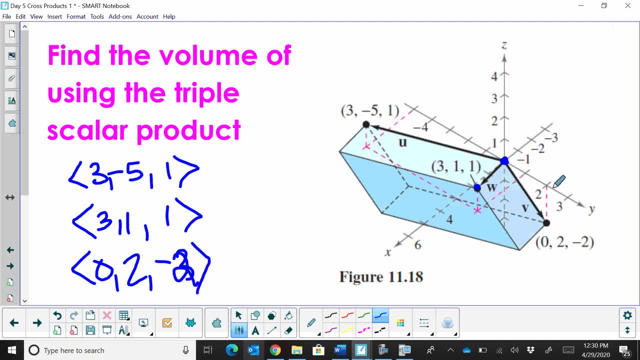 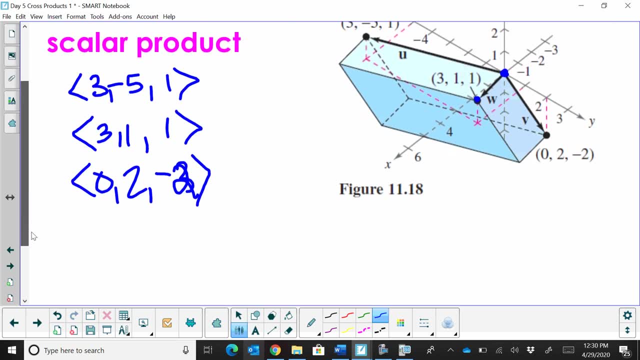 third. oops, that's a 2.. And it is the third side of this three-dimensional figure. So there are our three vectors that represent the three sides. We're going to set those up in a 3 by 3 matrix, So we're just going. 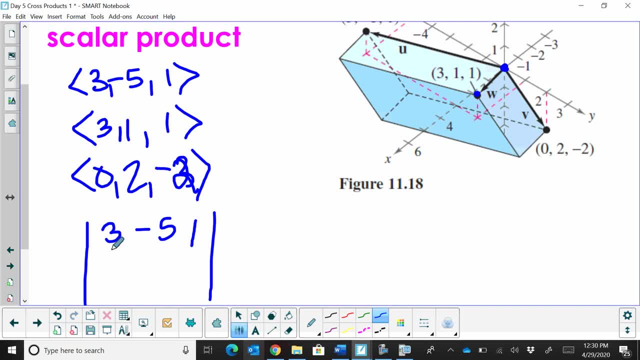 to set them up as 3, negative 5, 1.. Each one is a row: 3, 1, 1.. And 0, 2, negative 2.. Then we're going to grab our calculators And we're going to go to our matrix. 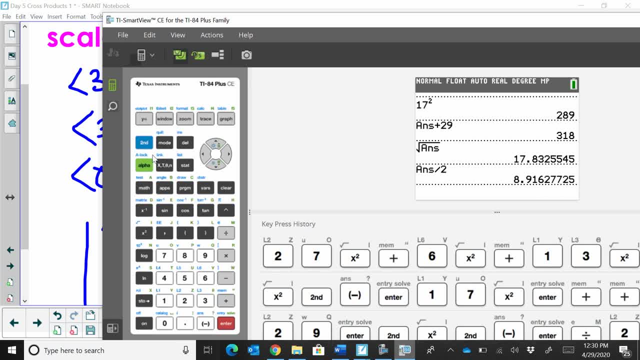 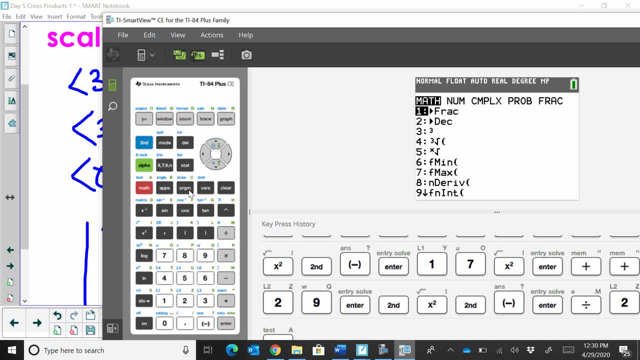 Now, it's been a while since I've done a matrix, So let's see. Our matrix is. where is our matrix Here? it is Second x to the negative 1.. We are going to go over and edit. Okay, The first thing I'm going to do is edit my matrix A and it's already set up as a. 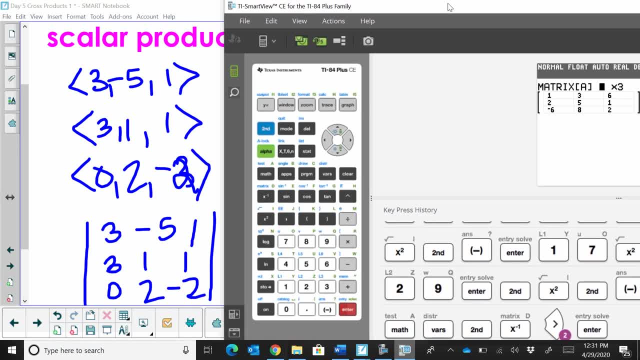 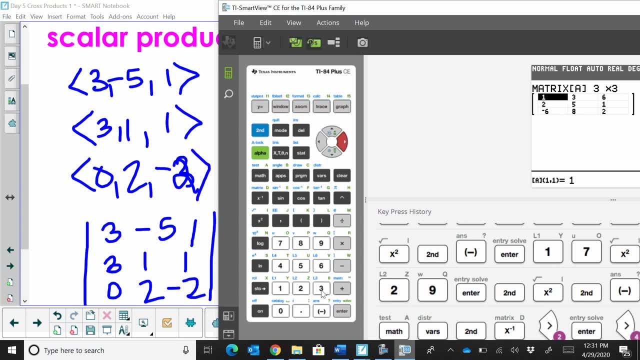 three by three. So it's nice. I'm going to now enter my new matrix. So I go down to the first entry and I enter three, enter negative five enter one, enter. And it goes to the second row, which is three enter one, enter, one, enter. And then it goes to my third row: zero enter. 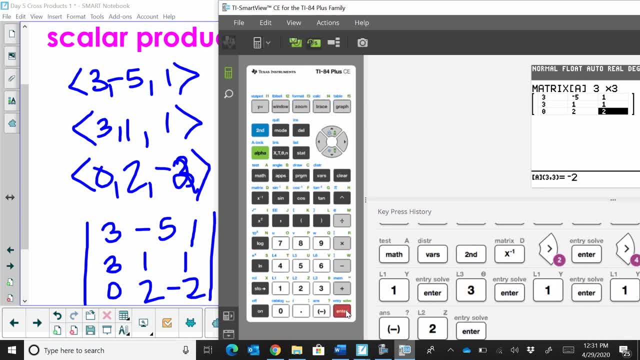 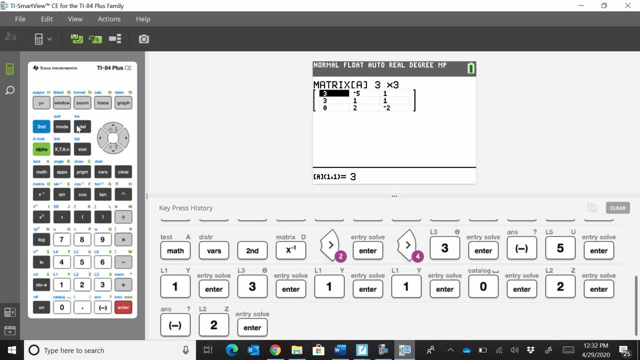 two enter and then negative two enter. So I've got my matrix in matrix A. Now I want to find my determinant. So I'm going to quit and go back to my home screen. And now let's find the determinant. 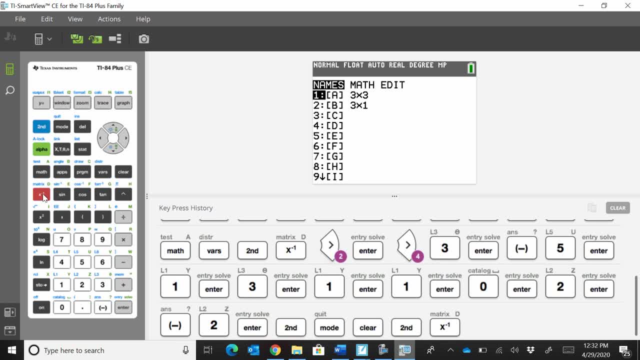 So I'm going to do second x to the negative one And I want to go over to the math key. The very first choice under here is determinant. So I'm going to enter that onto the home screen and do second matrix And I have. 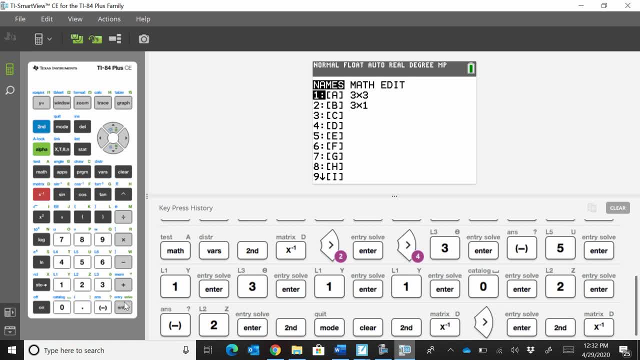 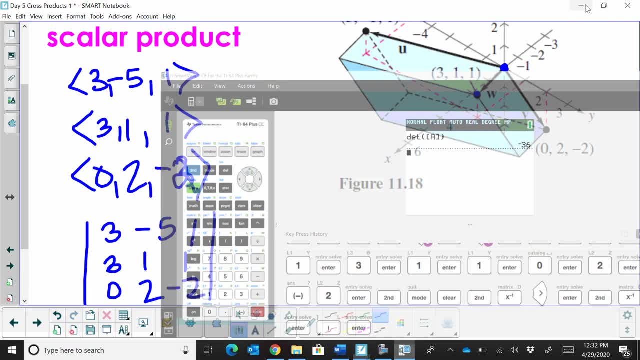 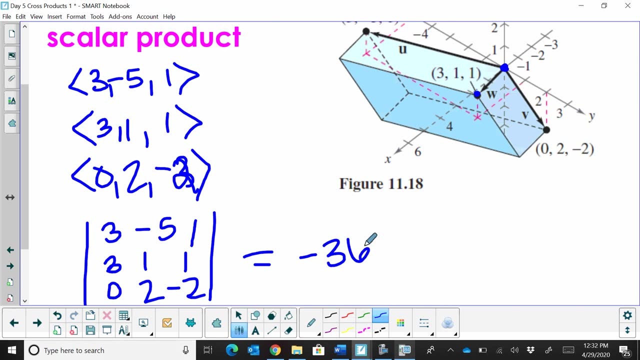 entered my information, the matrix I want in A, So enter yet again and find the determinant, which is negative 36.. Now that is the determinant of this matrix. Now that doesn't mean the volume is negative 36.. I'm going to take the absolute value of. 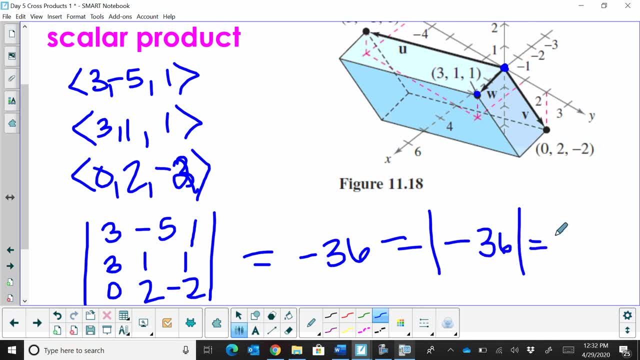 that determinant and that gives me the volume of my parallel pipe. So it's 36 units squared. So although the determinant is negative, you just take the absolute value of it and that is the you now. had I entered these in a different order, I might have gotten a positive 36. so really it just 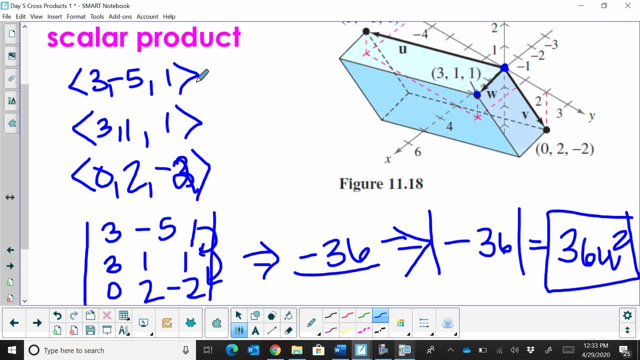 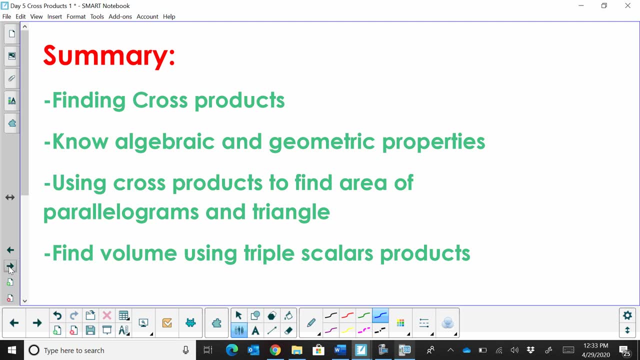 has everything to do that with the order that you put these in. so it doesn't matter what order you put them in, but each row is a vector and it's very, very simple, okay, so in summary, we have found, we identified finding cross products in the first video and we looked at the algebraic properties. 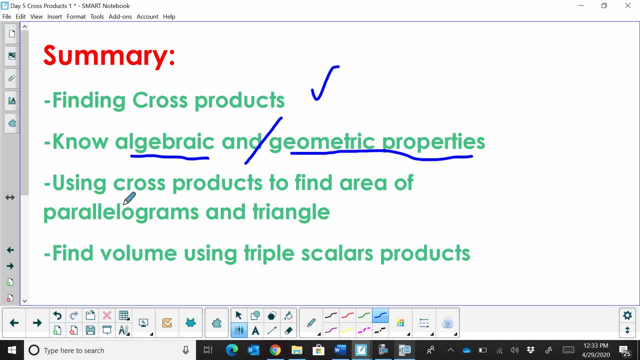 in the second video we looked at the geometric properties, how to use cross products to find the area of a parallelogram and a triangle. and that's when you use the IJK on the first row and then plug in your vectors on the second and third row, find the resulting cross product. 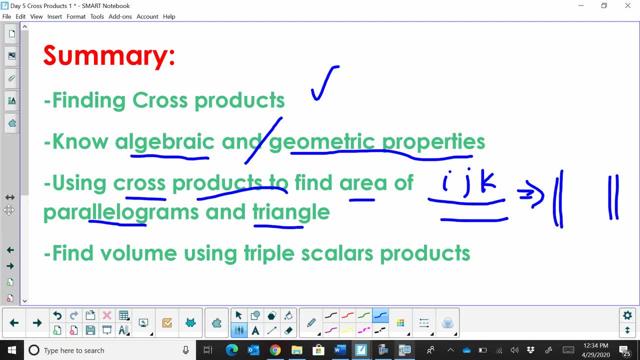 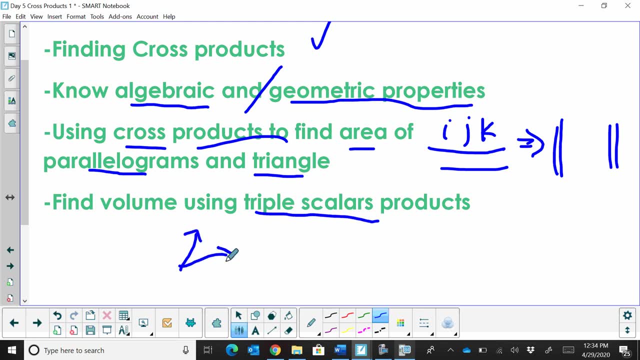 and then find the magnitude of that one, and then for the volume of a triple scaler. so when you have three vectors- one, two, three- you can find the volume of that 3d figure by simply using a matrix, a three by three matrix, to find the determinant. and then, of course, once you find that determinant, 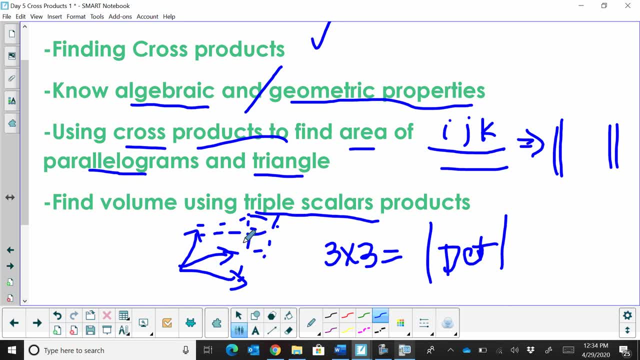 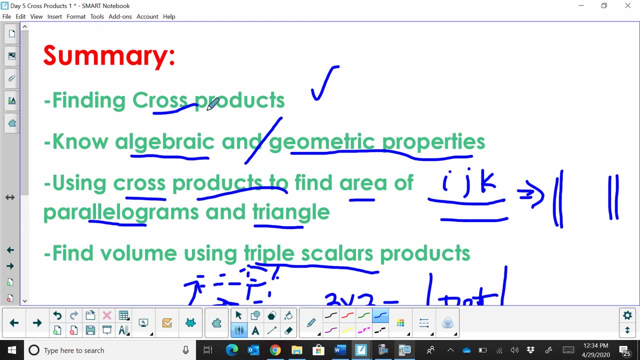 you take the absolute value of it, and that's it That represents the volume of the 3D figure, which we call a parallel pipe. So there we go. That's the end of this set of lessons on cross products for vectors in three dimensions.